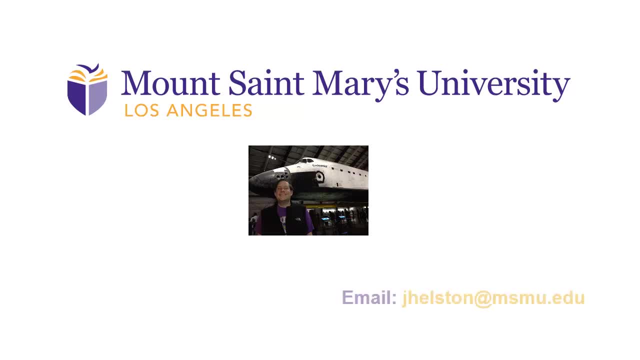 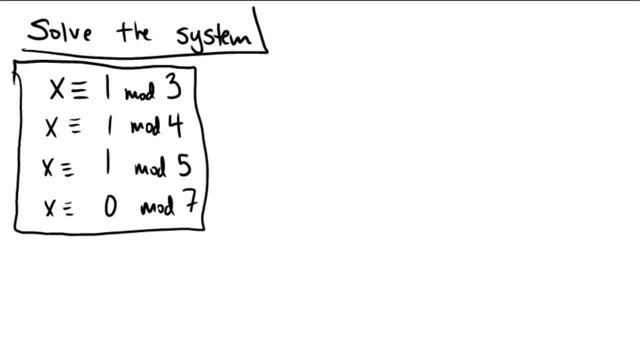 Okay, here we're going to solve a system of congruences using the Chinese Remainders Theorem. So x is congruent to 1, mod 3, mod 4, mod 5, and it's congruent to 0, mod 7.. 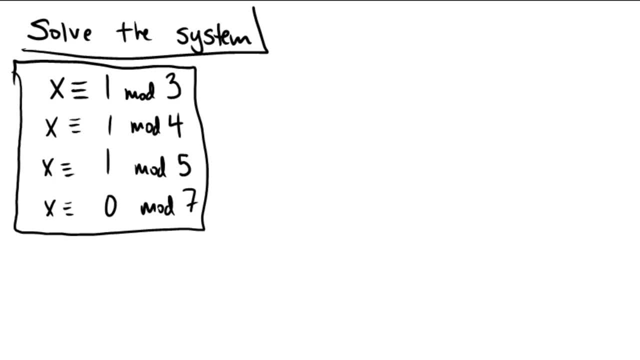 So since 3,, 4,, 5, and 7 are pairwise, relatively prime, there's no common factors amongst any of them, I can use the Chinese Remainders Theorem to solve this problem. So for the Chinese Remainders Theorem, first of all, 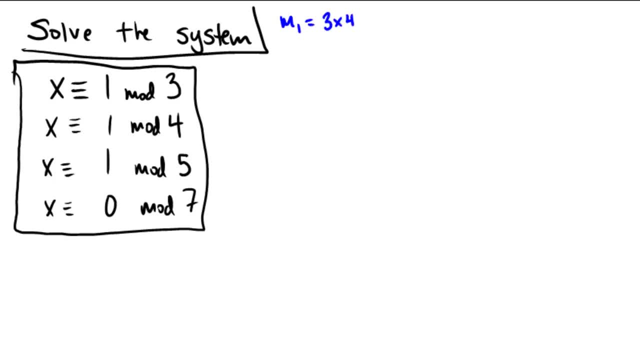 m1 is equal to 3 times 4 times 5 times 7, which is equal to 420, which means we'll find a unique solution up to mod 420.. We'll find an answer less than 420.. Okay, that's our little m. 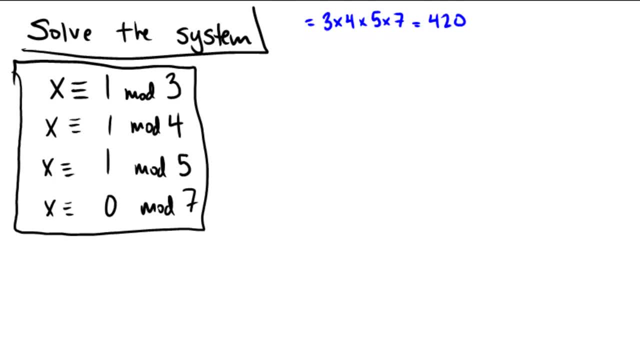 Actually, I shouldn't even put a subscript on that one. Just Little m, The product of all of these pieces. Okay, now the process is to find capital M1,, which would be the product of the other ones that are not 3.. 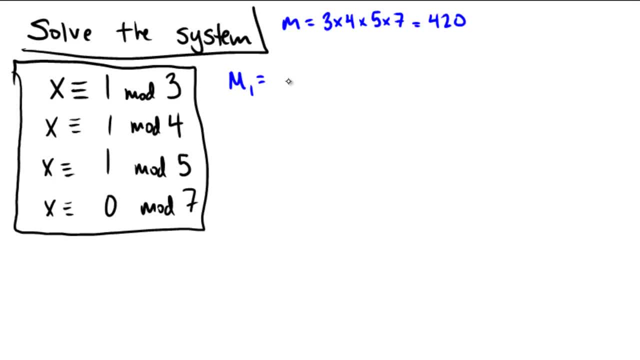 So 4 times 5 times 7.. 4 times 5 times 7.. So, not the 3, would be 140.. M2 is 3 times 5 times 7.. Everything but the 4. So that would be 105.. 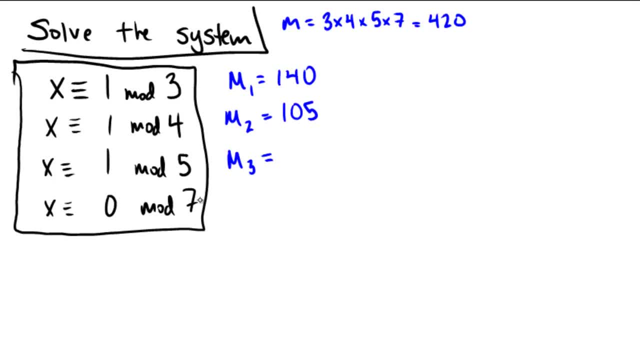 M3 is 3 times 4, is 12 times 7,, which is 84.. And then M4 would be 3 times 4 times 5, which is just 60.. So that's M1, M2, and M3, and M4. 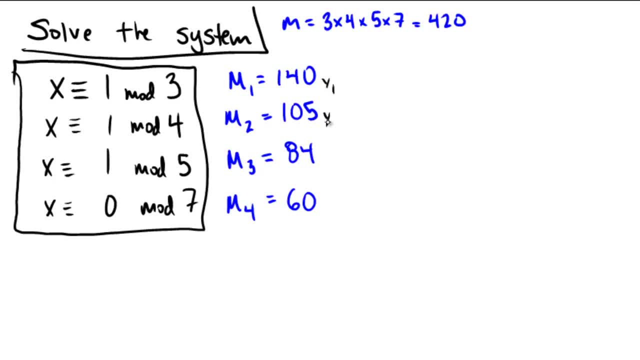 Okay, the next step of the problem is to find numbers y1, y2, y3, y4, which multiply by those numbers there, all of which are meant to be congruent to 1, 1 mod the respective base. 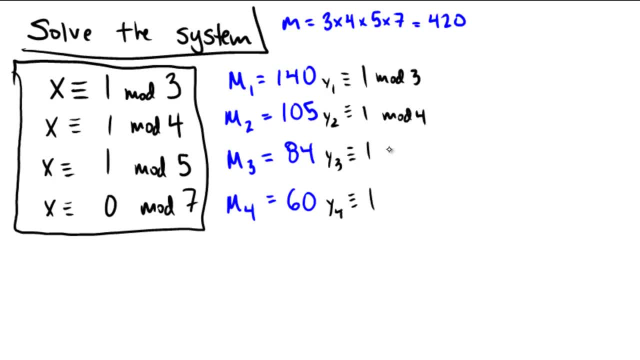 So this would be 1 mod 3.. This would be 1 mod 4.. This would be 1 mod 5.. And this would be 1 mod 7.. Now, fortunately, since 3,, 4,, 5, and 7 are so small, 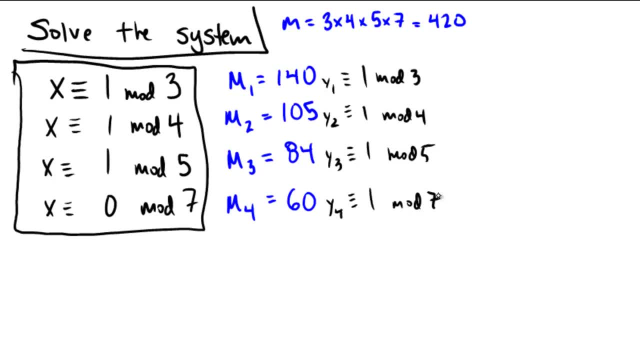 we should be able to do this kind of mentally, But if you didn't have that opportunity, then you might need to use the Euclidean algorithm to find the inverses. Okay, but we can do this pretty straightforward here, I think. So, first of all, 140 is gigantic. 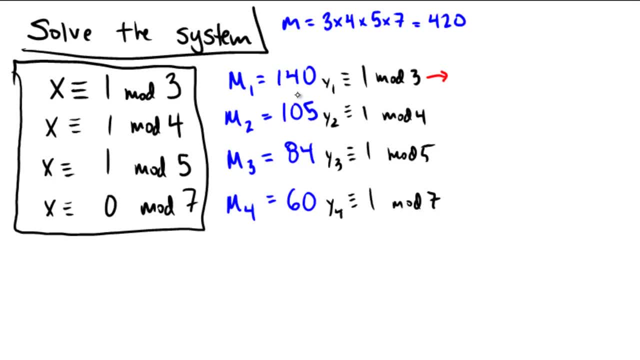 Compatible Compared to mod 3.. So let's reduce that mod 3 first, And if you take 140, let's see 138 is a multiple of 3, so a remainder of 2.. So we actually have 2y1 being congruent to 1 mod 3.. 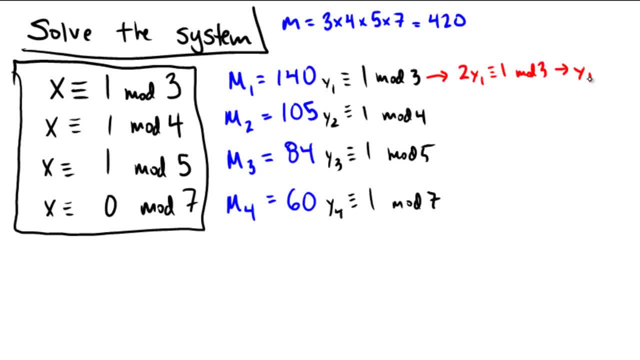 And so that would mean that y1,. let's see, it wouldn't be 1, because 2 times 1 is not 1, but it would be y1 would be equal to 2, because notice that 2 times 2 is 4,. 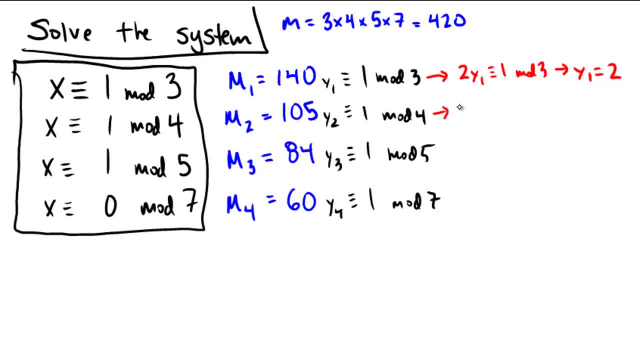 which is congruent to 1 mod 3.. Okay, next row to find y2.. 105 reduced mod 4.. Turns out, 104 is a multiple of 4, so this would just be the same as 1y2 is congruent to 1 mod 4.. 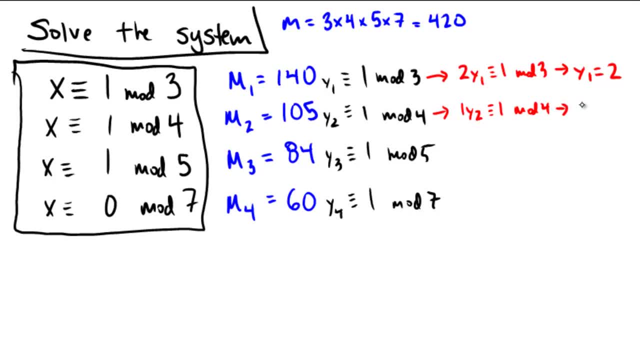 And that's really convenient, because that's just 1, right, The 1 is just 1.. So y2 can just be equal to 1.. Okay, next one: 84, mod 5.. Let's see, 80 goes in 16 times 5 is 80,. 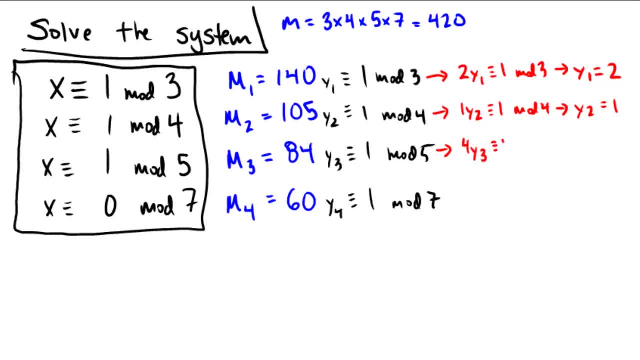 so this leaves with 4.. y3 congruent to 1 mod 5, which means that we have to find a number less than 5. that gets me up to the right place with the 4.. I'm using a little strategy here: that 4 is 1 less than 5,. 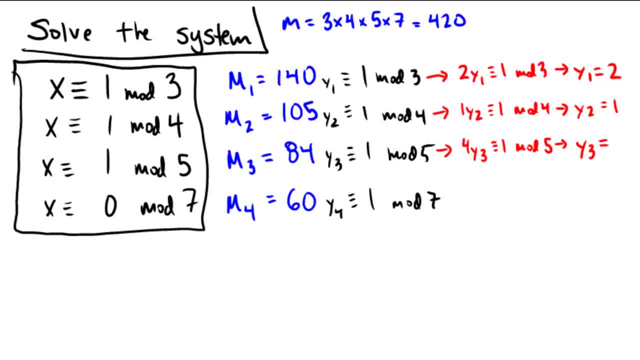 so it's equivalent to negative 1.. So I know that y3 is just going to be 4 again, because negative 1 times negative 1 is 1.. But just think: 4 times 4 is 16, and 16 mod 5 is clearly 1.. 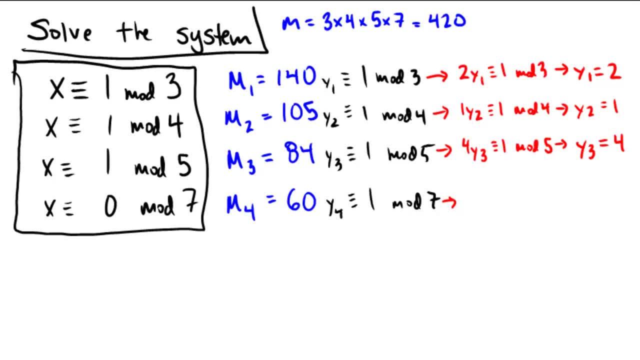 Okay, one more to go here. The last one is mod 7 on 60, so 8 times 7 is 56, so I'm going to get a 4 multiplied by a y4 needs to be congruent to 1 mod 7.. 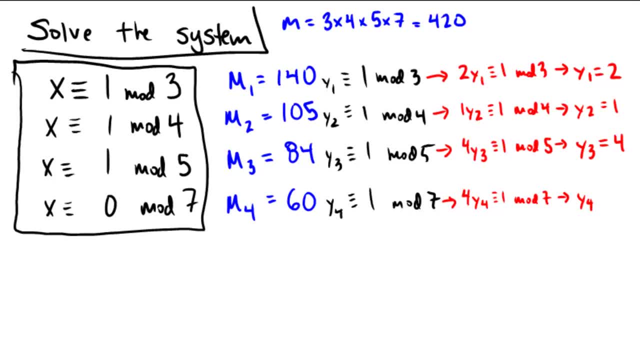 And that means that y4 is going to have to be. let's see, 4 doesn't work. 4 times 2 is 8.. Oh yeah, 8 is remainder 1 mod 7, so this will just be a 2, because 4 times 2 is 8..